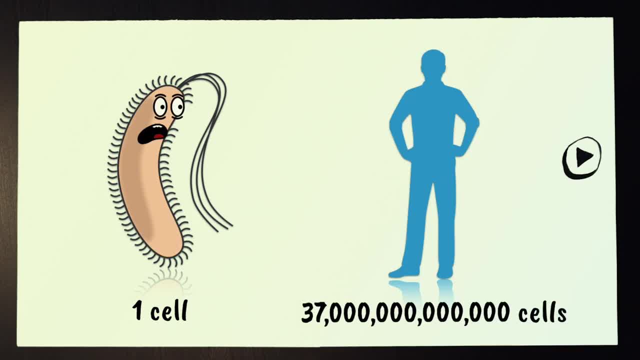 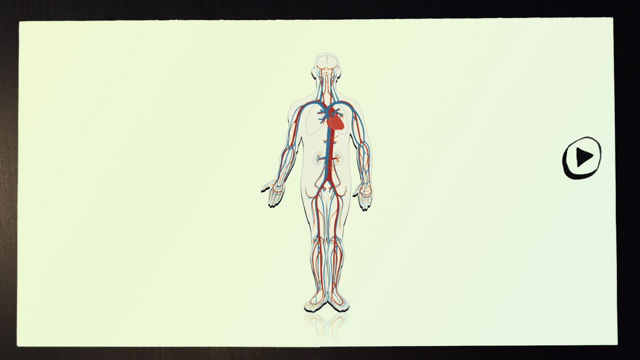 up of millions of cells. To get the important stuff, like oxygen, to all of the cells that make up our bodies, we have a transport system that take things to where we need them. We rely on the blood to transport what we need to where we need it. 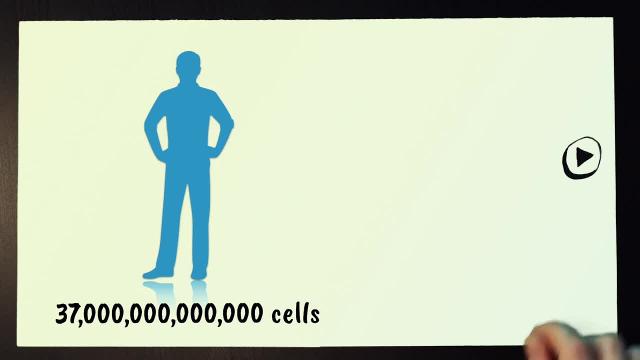 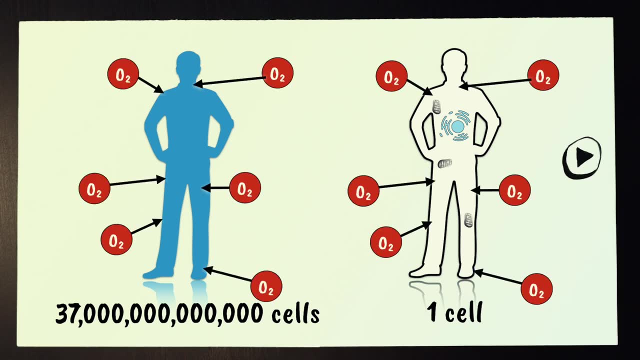 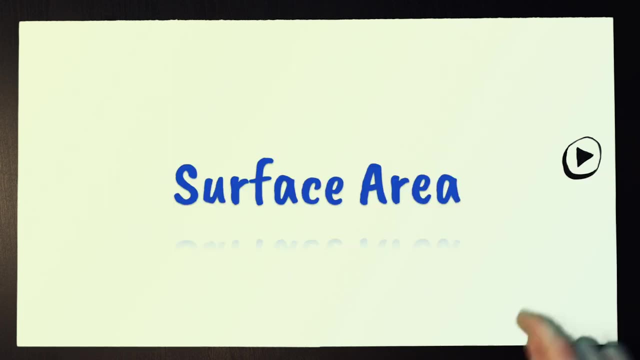 But why are larger organisms made of many cells rather than a single giant cell, And why do we need such advanced transport systems rather than simply allowing materials like oxygen to diffuse? The problem is surface area. Consider two cubes of different sizes. The smallest cube. 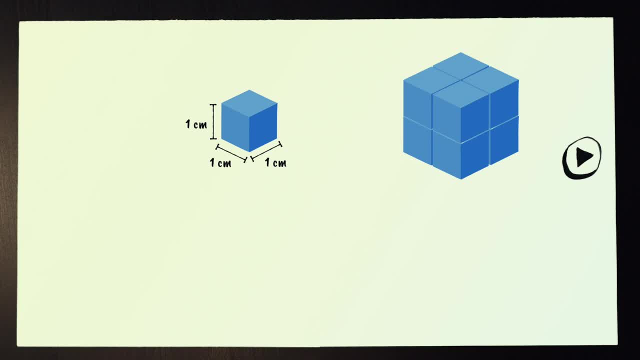 is 1cm by 1cm by 1cm, and so it has faces, each with an area of 1cm squared, And there are six faces, so it has a total surface area of 6cm squared. The larger cube is 2cm by. 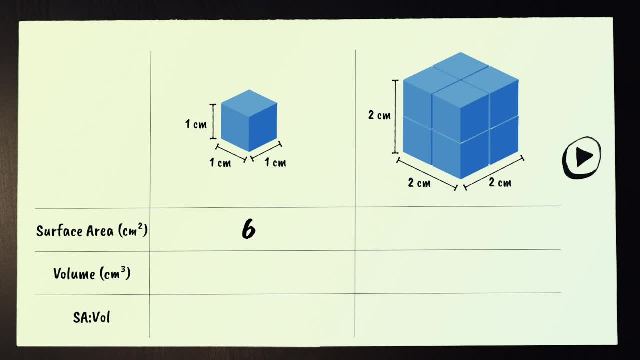 2cm by 2cm, So it has a total surface area of 6cm squared, And so it has a total surface area of 6cm by 2cm, So each face is 4cm squared. With six faces, it has a total surface area. 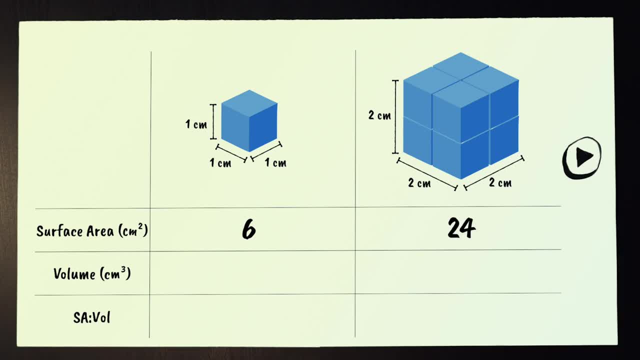 of 24cm squared. So the larger cube has a larger surface area. but the larger cube also has a larger volume. We need to compare the surface area of each cube with its own volume. The small cube has a volume of 1 by 1 by 1, which is 1cm cubed. It has 6cm2 of surface. 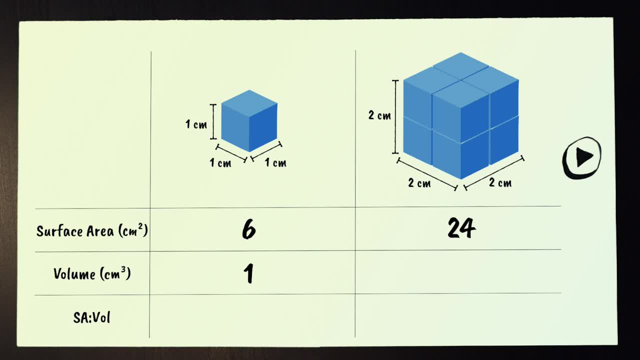 area for every 1cm, We can say that it has a surface area to volume ratio of 6 to 1.. If we do the same for the larger cube, we can say that it has a volume of 2 times 2 times 2, which equals 8cm cubed. 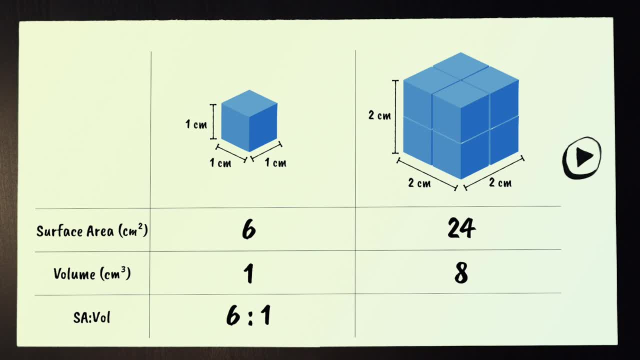 This ratio of 24cm2 of surface area to every 8cm2 of volume can be simplified to 3 to 1.. 6 to 1 is bigger than 3 to 1.. It's obvious that the smaller cube has a volume of 1 by. 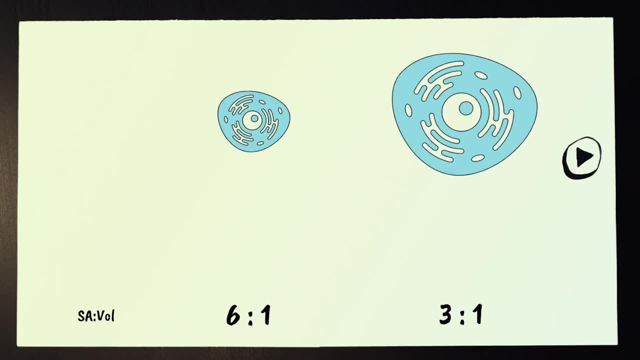 1. The larger cube has a larger surface area to volume ratio. Let's imagine that these cubes are living cells that need oxygen to survive. For oxygen to spread throughout the cells, it must diffuse through the surface. As the small cell has more surface area relative to its volume, every part of that volume can be supplied.